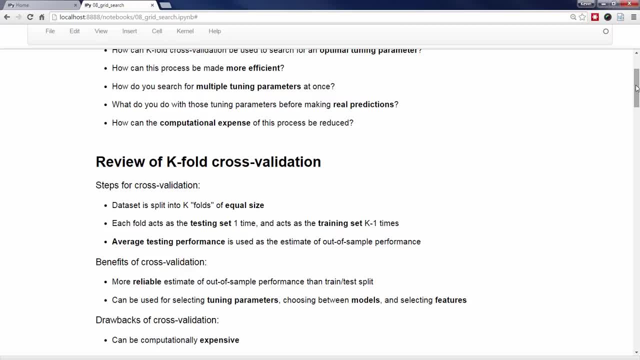 The average testing performance, also known as the cross-validated performance, is used as the estimate of the model's performance on out-of-sample data. That performance estimate is more reliable than the estimate provided by train-test-split because cross-validation reduces the variance associated with a sample. 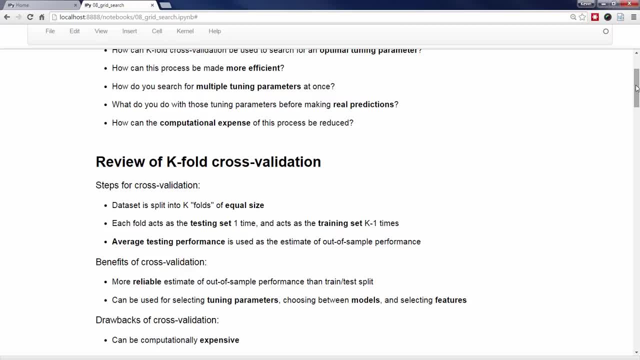 This is associated with a single trial of train-test-split, As we saw in the last video. cross-validation can be used for selecting tuning parameters, choosing between models and selecting features. However, cross-validation can be computationally expensive, especially when the dataset is very large or the model is slow to train. 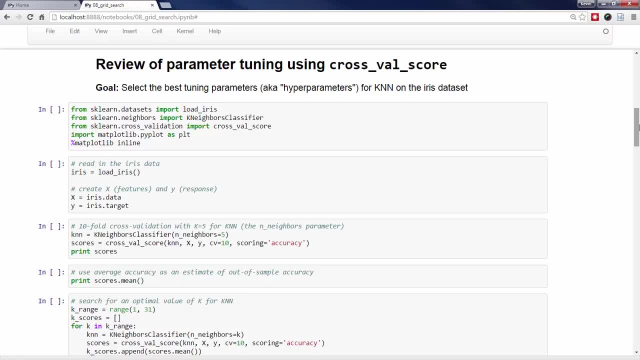 There is no standard or standard of tuning for cross-validation. Let's now review how we used the cross-val score function in the last video to select the best tuning parameters. It's important to understand this code because it will help you to understand the role of grid search CV, which I'll be covering in the next section of this video. 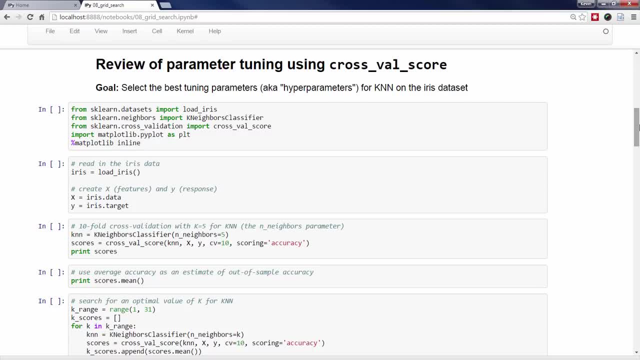 In this case, we were trying to select the best value for k model when predicting species on the iris dataset. We'll start by importing the relevant functions and classes and then creating the feature matrix x and response vector y. Next, we'll instantiate the k-neighbors classifier with a k value of 5, represented. 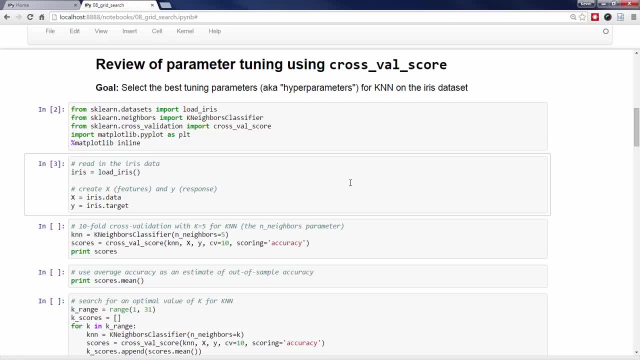 by the n-neighbors parameter. The model object, which we called knn, is used as the first parameter in CrossValScore. The other four parameters are the feature matrix x, the response vector y, the number of cross-validation folds to use and the evaluation metric of our choice. 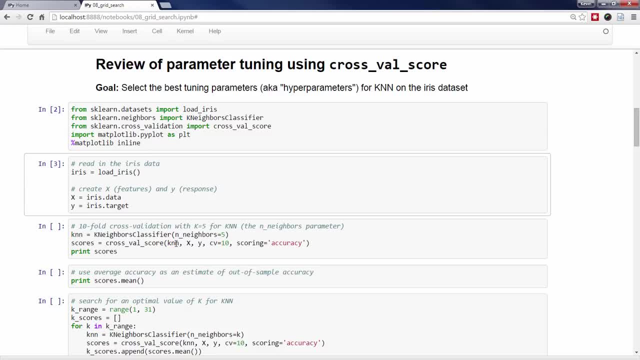 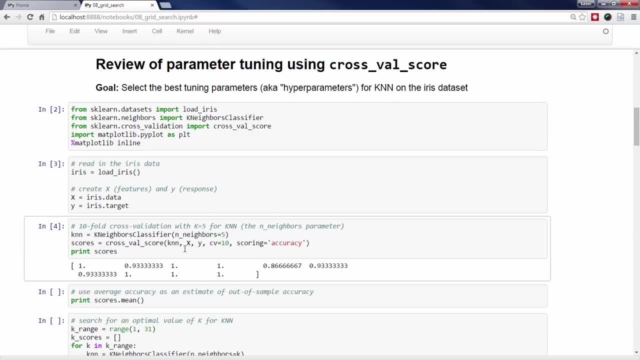 We're choosing to use tenfold cross-validation. CrossValScore returned ten scores, namely the testing accuracy for each of the tenfolds used during cross-validation. Remember that CrossValScore takes care of the entire cross-validation process, including splitting x and y into the tenfolds. 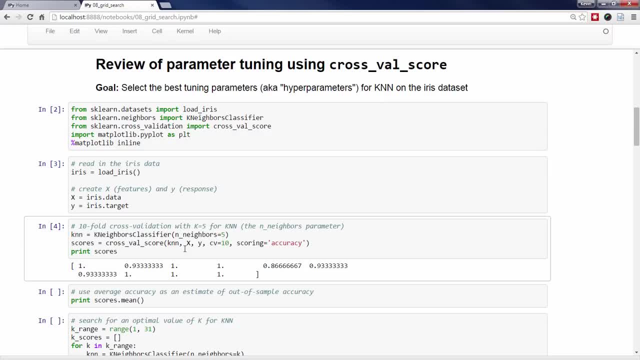 We're going to use the cross-validation method for this. CrossValScore is the first parameter in CrossValScore, which is why we passed it the entirety of x and y and not x-train and y-train. The scores object is a numpy array, and so we can use its mean method in order to calculate. 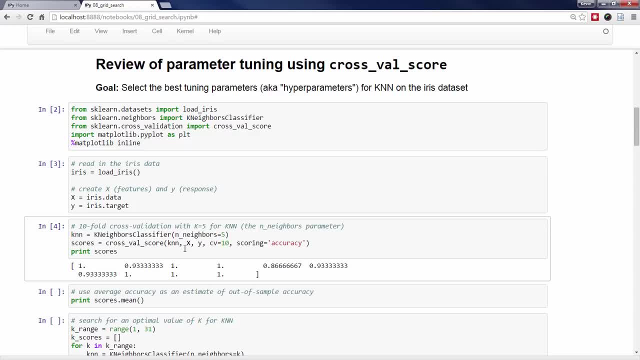 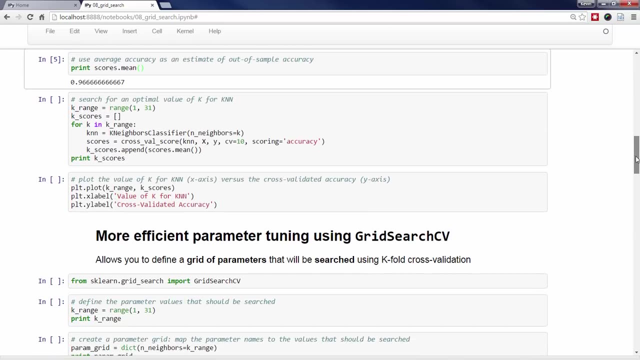 the mean which we use as the estimated accuracy for the k equals 5 model on the iris dataset. We want to repeat this process for a variety of k values. to choose the k which will most likely generalize to out-of-sample data, and thus using a for loop, is a natural choice. 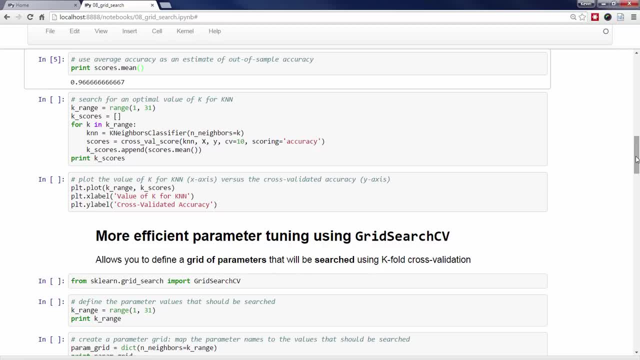 Pay close attention here, because this is the code that we're going to replace with GridSearchCV. We start by creating two lists: kRange contains the integers 1 through 30, and indicates the values of k that we want to try, and kScores is an empty list that will be used to store the cross-validated 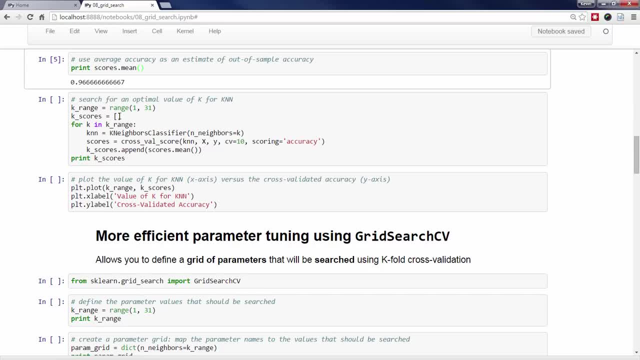 accuracy for each of the 30 iterations. The for loop iterates through kRange and within the loop we instantiate kNeighborsClassifier with the chosen k value, use CrossValScore to perform tenfold cross-validation and then append the mean of the 10 scores to the kScores list. 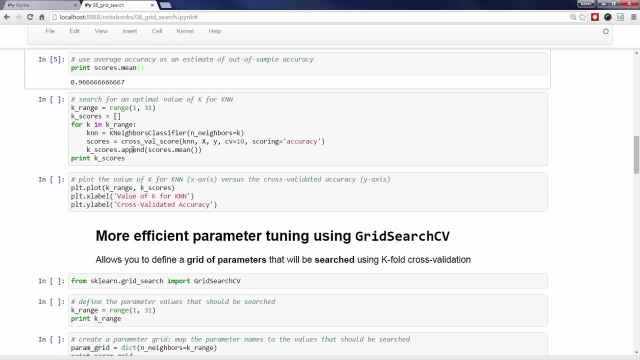 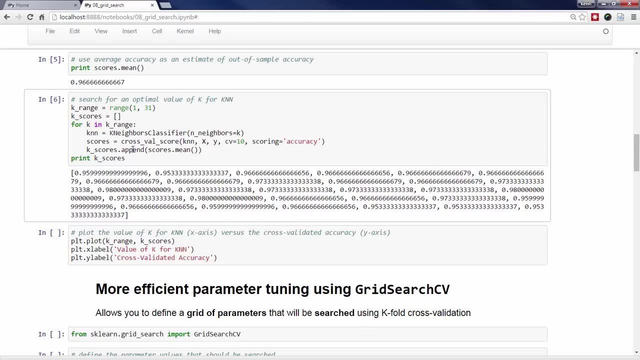 Finally, we'll print the 30 cross-validated scores. As you would expect, the fifth score in this list is 0.96.. 0.966, which we knew from above, would be the cross-validated score when nNeighbors. 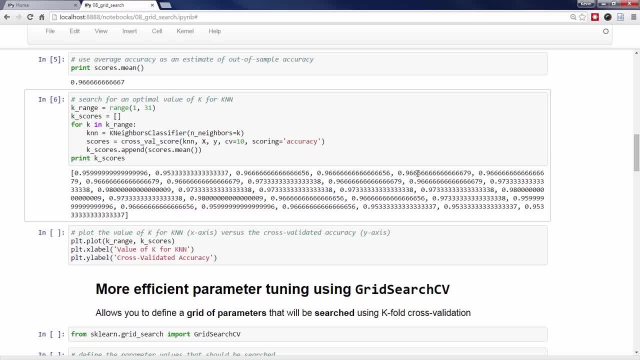 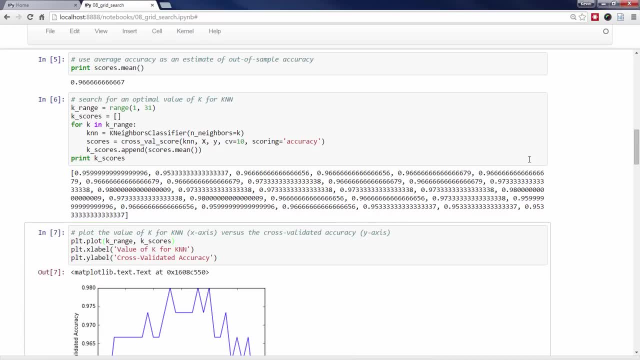 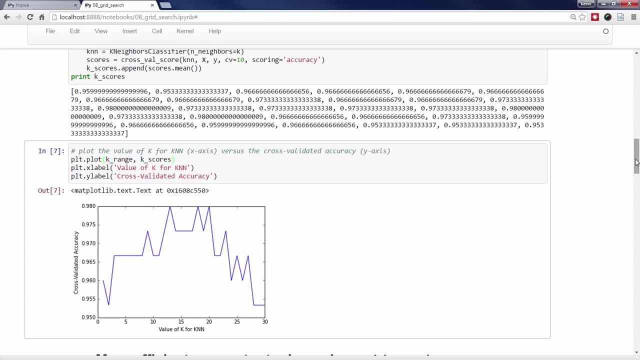 equals 5.. Finally, we plot the k values against the accuracy. We see that the values 13,, 18, and 20 for k appear to be best. We see that our ofKneighbors' return at trials is 10.. 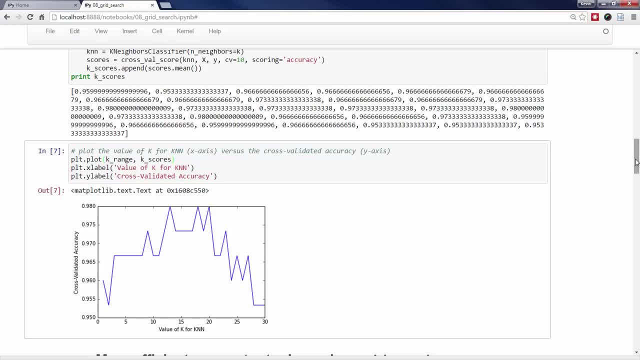 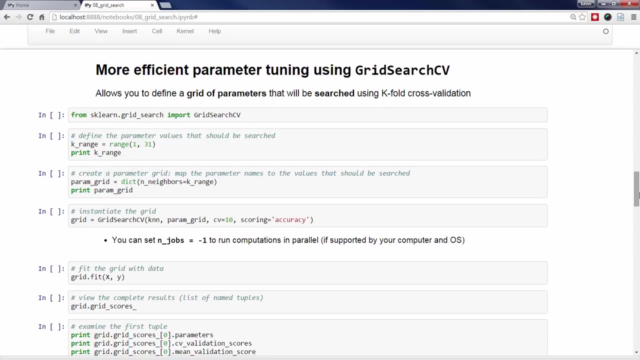 Even though the above is not particularly difficult to write, you could imagine that this is something you might want to do very often, and thus it would be nice if there is a function that could automate this process for you. That's exactly why GridSearchcv was created. 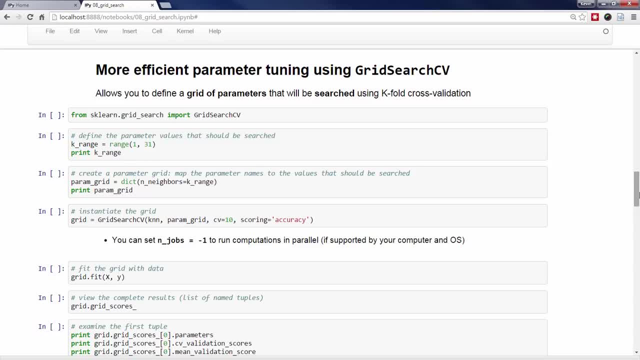 Look at this set of parameters that you want to try with a given model, and it will automatically run cross-validation using each of those parameters, keeping track of the resulting scores. Essentially, it replaces the for loop above, as well as providing some additional functionality. 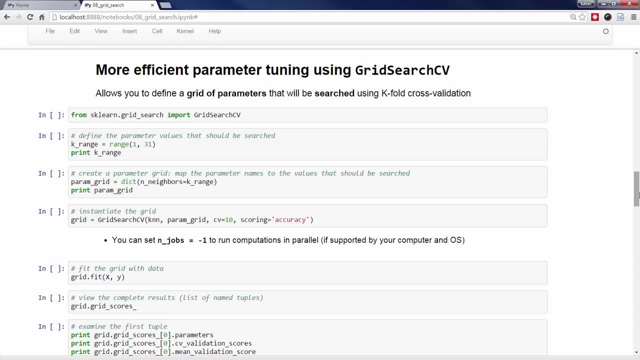 To get started with GridSearchCV, we first import the class from sklearngridsearch. Exactly like above, we create a Python list called kRange that specifies the k values that we would like to search. Next, we create what is known as a parameter grid. 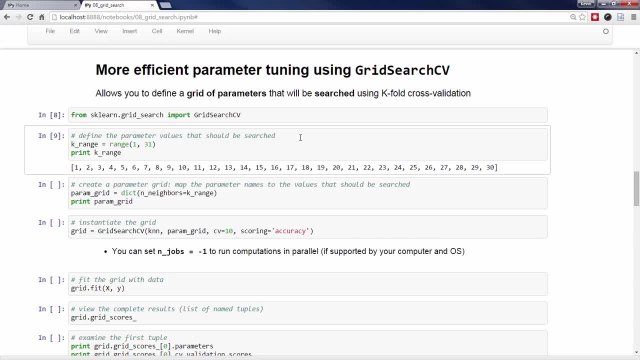 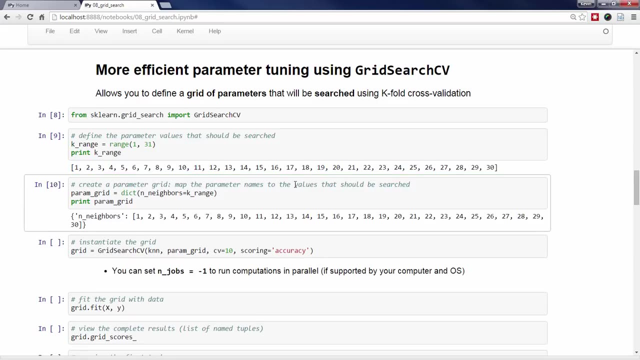 It's simply a Python dictionary in which the key is the parameter name and the key is the parameter name And the value is a list of values that should be searched for that parameter. As you can see, this dictionary has a single key-value pair in which the key is the string. 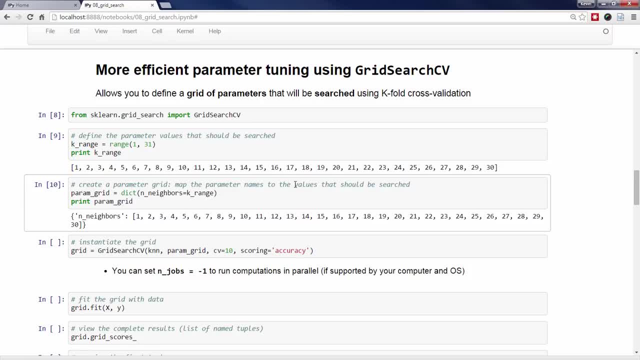 and neighbors, and the value is a list of the numbers 1 through 30.. Next we'll instantiate the grid. You'll notice that it has the same number of values as the string and neighbors, but it has the same parameters as CrossValScore, except that it doesn't include x or y. but 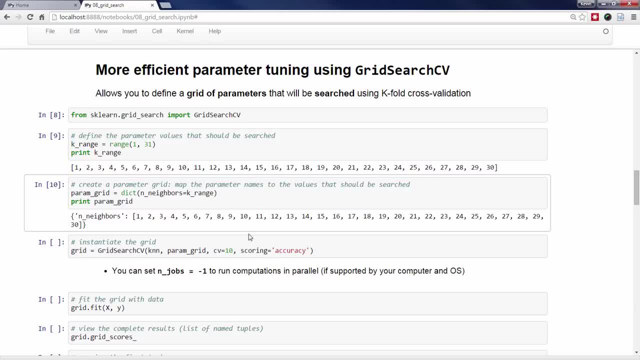 it does include ParamGrid. You can think of the grid object as follows: It's an object that is ready to do tenfold cross-validation on a KNN model, using classification accuracy as the evaluation, But in addition it has been given this parameter, grid, so that it knows that it should repeat. 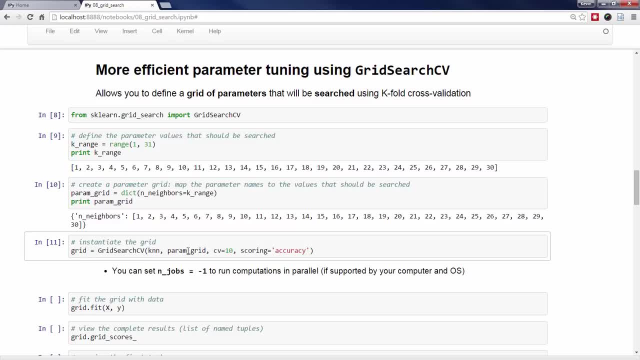 the tenfold cross-validation process 30 times, and each time the NNeighbors parameter should be given a different value from the list. Hopefully, this helps you to understand why the parameter grid is so important to us. The grid is specified using key-value pairs. 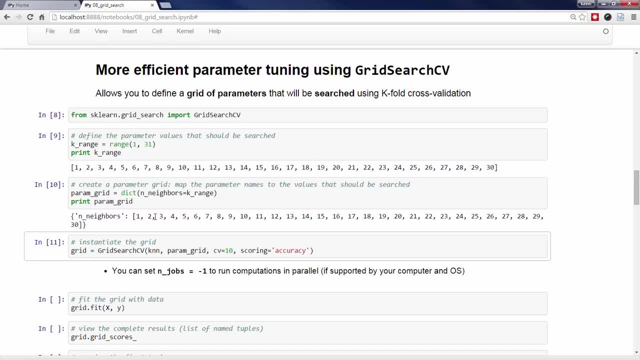 We can't just give GridSearchCV a list of the numbers 1 through 30, because it won't know what to do with those numbers. Instead, we need to specify which model parameter- in this case NNeighbors- should take on the 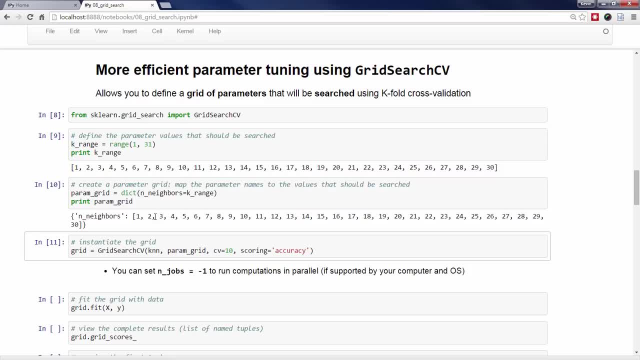 values 1 through 30.. One final note about instantiating the grid 1.. If your computer and operating system support parallel processing, you can set the njobs parameter to negative 1 to instruct scikit-learn to use all available processors. 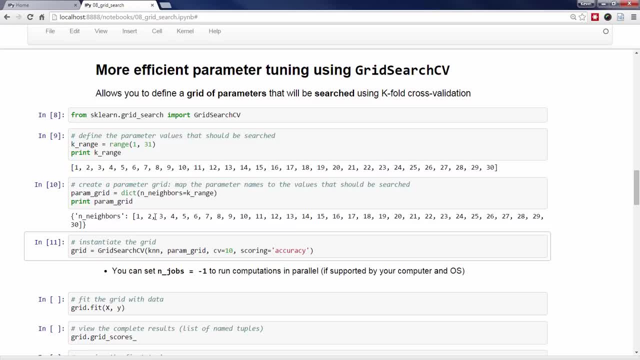 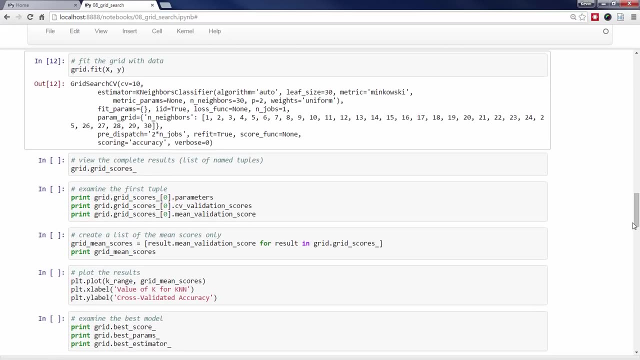 Finally, we fit the grid with data by just passing it: the x and y objects. This step may take quite a while, depending upon the model and the data and the number of parameters being searched. Remember that this is running tenfold cross-validation 30 times, and thus the KNN model is being fit. 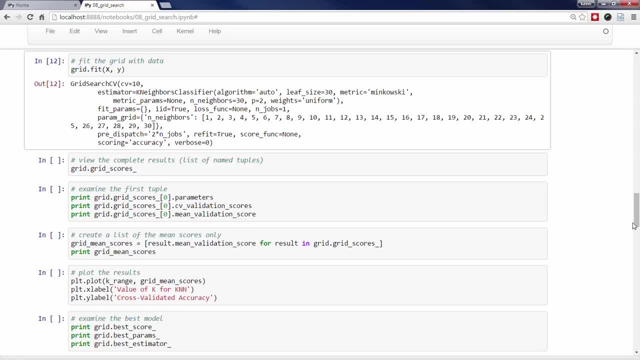 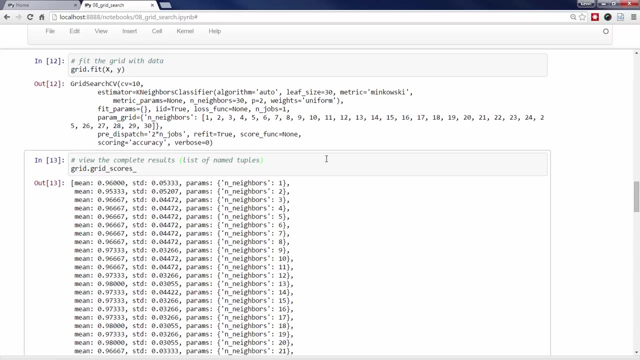 and predictions are being made 300 times. Now that grid search is done, let's take a look at the results, which are supposed to be in the grid scores attribute. This is actually a list of 30 named tuples. The first tuple indicates that when the NNeighbors parameter was set to 1, the mean cross-validated. 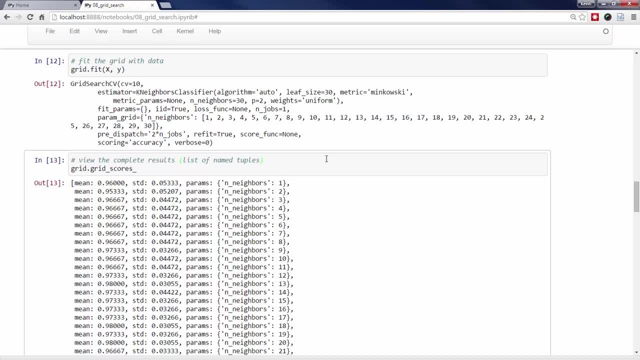 accuracy was 0.96, and the standard deviation of the accuracy scores was 0.05.. While the mean is usually what we pay attention to, the standard deviation can be useful to keep in mind because if the standard deviation is high, that means that the cross-validated 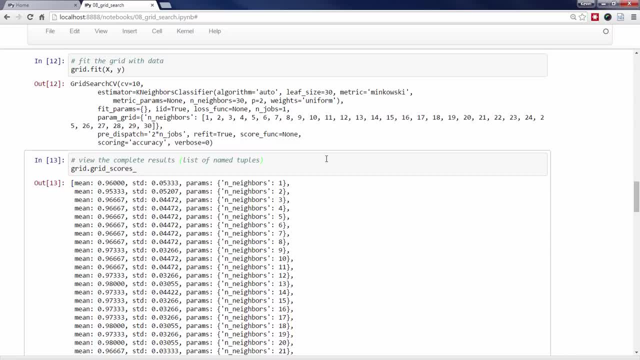 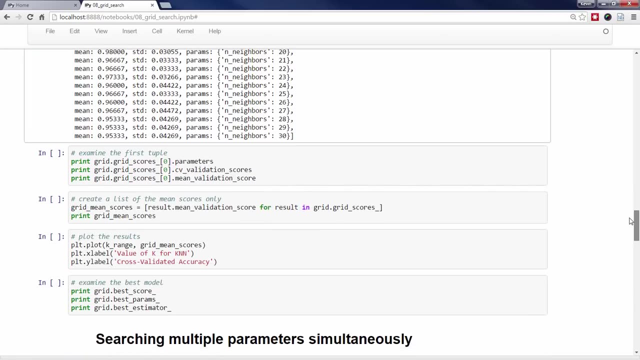 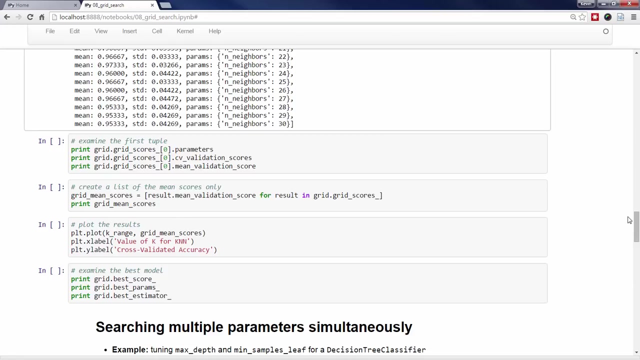 estimate of the accuracy might not be as reliable. Anyway, you can see that there is one tuple for each of the 30 trials of cross-validation. You can see that there is one tuple for each of the 30 trials of cross-validation. Next I'll just show you how you can examine the individual tuples, just in case you need. 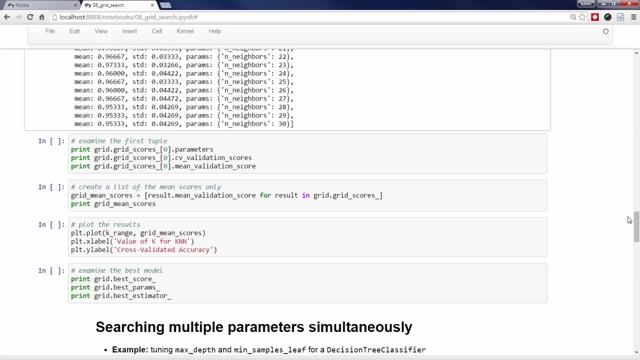 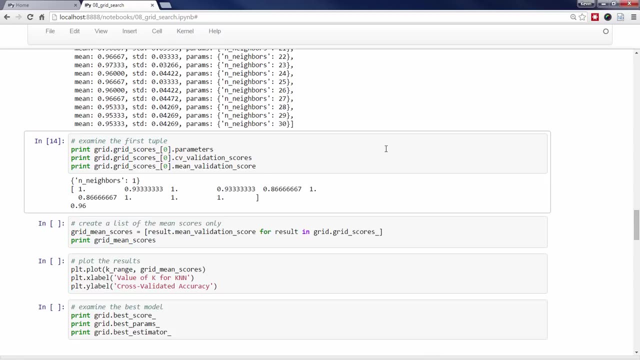 to do so in the future. I'm going to slice the list to select the first tuple using the bracket zero notation, Because it's a named tuple. I can select its elements using dot notation 1.. Parameters is simply a dictionary containing the parameters that were used. 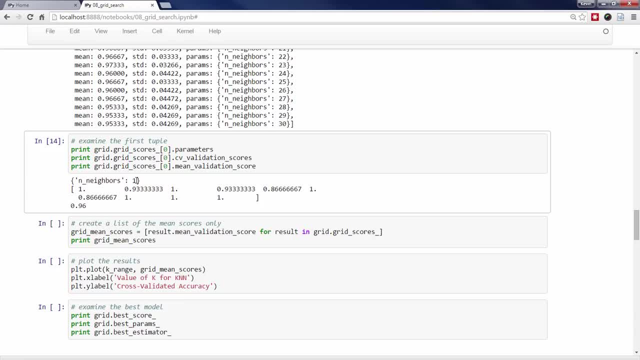 1. CvVal is an array of the 10 accuracy scores that were generated during ten-fold cross-validation using that parameter. 3. し and meanVal is, of course, the mean of those scores. 4. 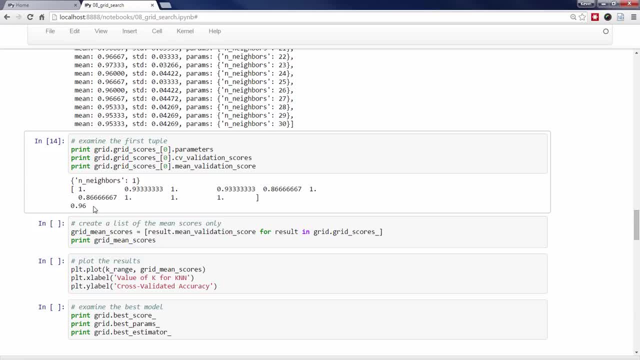 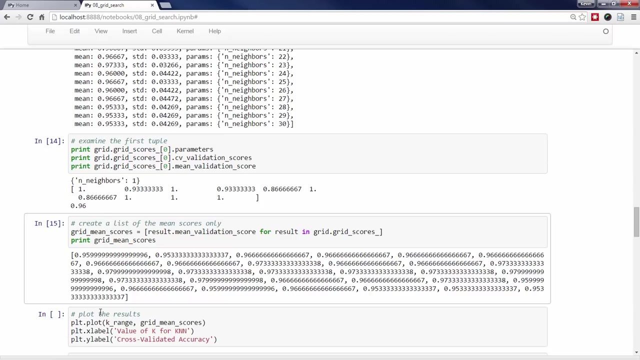 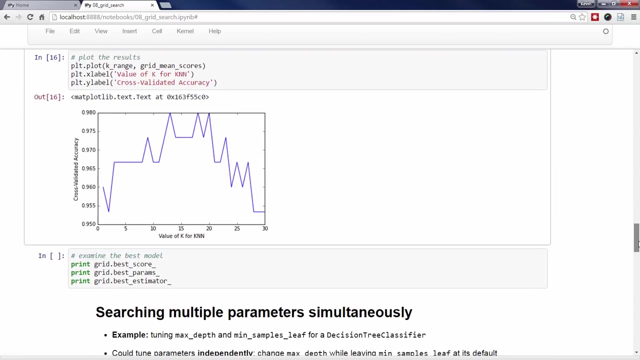 mean scores across the 30 runs and plot them like we did above. so let's just quickly do that. we'll use a list comprehension to loop through grid dot grid scores, pulling out only the mean score, and when we plot the results we can see that the plot is identical to the one we generated above. 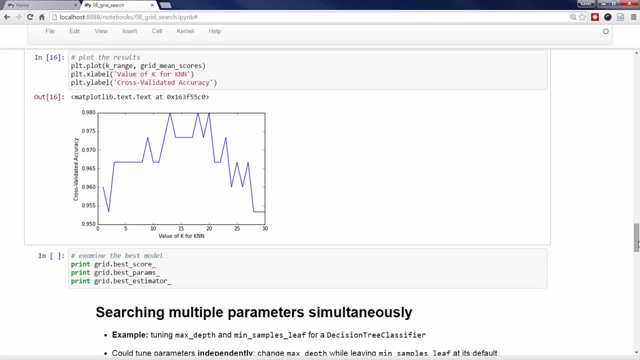 now you might be thinking that writing a list comprehension- and then making a plot can't possibly be the most efficient way to view the results of the grid search. you're exactly right. once a grid has been fit with data, it exposes three attributes that are quite useful. 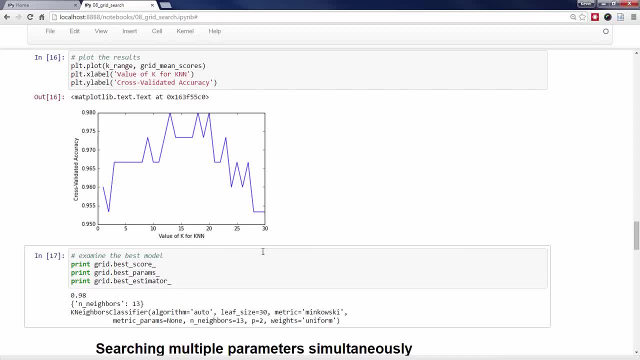 best score is the single best score achieved across all of the parameters. best params is a dictionary containing the parameters used to generate that score. and finally, best estimator is the actual model object fit with those best parameters, which conveniently shows you that the best score is the single best score. 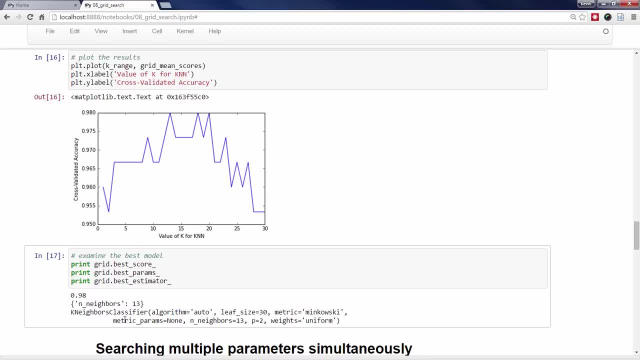 and that the best score is the single best score and that the best score is the single best score and that the best score is the single best score. as you might have noticed in the plot, there are two other values for k, which also produced a score of 0.98. i don't know for sure how grid search decided to choose k equals. 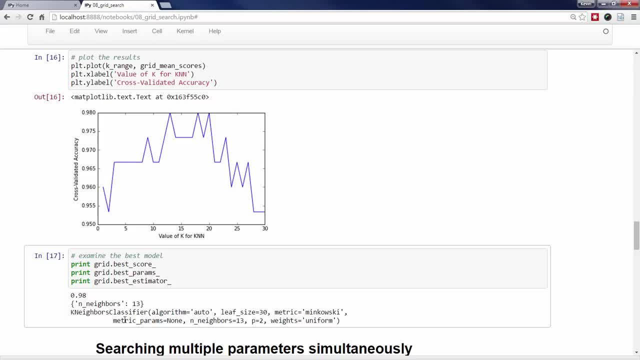 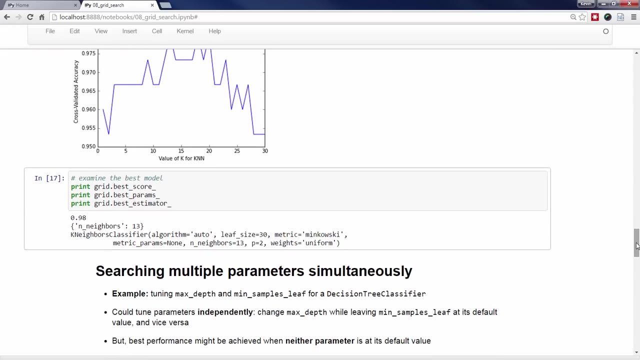 13 as the best, but some limited testing indicates that it probably just picks the first parameter it tested that achieved that score. it might have occurred to you already that sometimes you'll want to search multiple different parameters simultaneously for the same model, for example. let's pretend 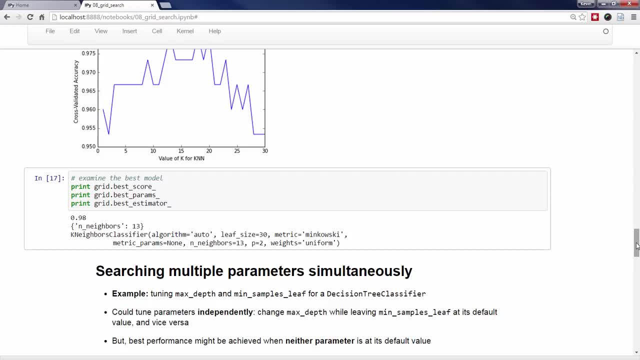 you're using a decision tree classifier, which is a model we haven't yet covered in the series. two important tuning parameters are max depth and min samples leaf. you could tune those parameters independently, meaning that you try different values for max depth while leaving min samples leaf at its default value, and then you try different. 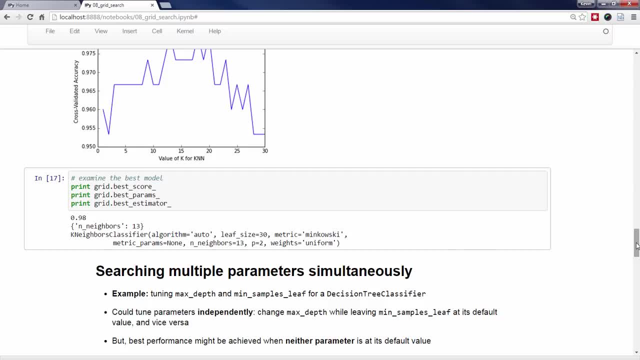 values for min samples leaf, while leaving max depth at its default value. the problem with that approach is that the best model performance might be achieved when neither of those parameters are at their default values. thus, you need to search those two parameters simultaneously, which is exactly what we're about to do with grid search cv. 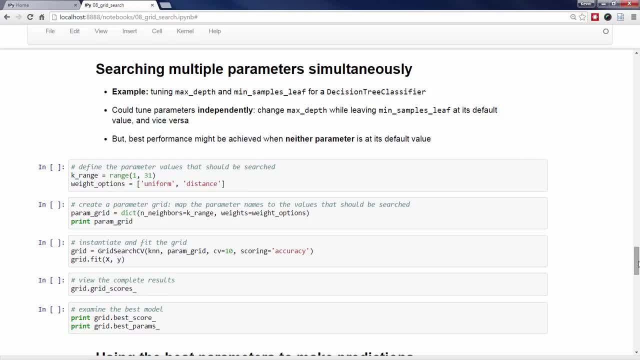 in the case of k and n. another parameter that might be worth tuning, other than k, is the weights parameter, which controls how the k nearest neighbors are weighted. when making a prediction, the default option is uniform, which means that all points in the neighborhood are weighted equally, but another option is distance, which weights closer neighbors more heavily than further neighbors. 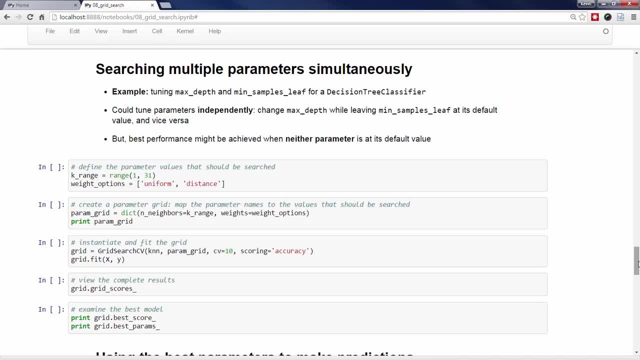 thus, i'm going to create a list of those options called weight options, in addition to the 30 integer options in k range. again, i create a parameter grid, which is 63, and because the dictionary has two key value pairs, one pair for each parameter to be, 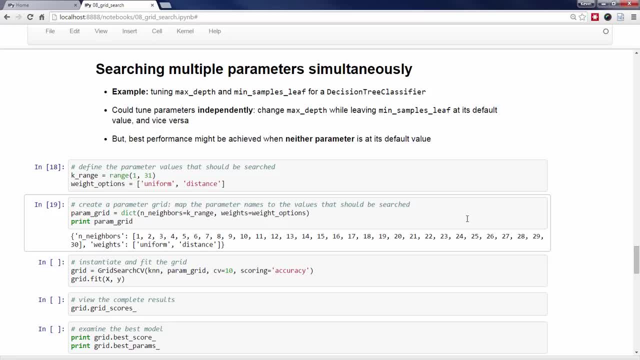 searched. now i'll instantiate the grid and fit it with data just like before. this is known as exhaustive grid search because grid search cv is trying every possible combination of the end neighbor's parameter and the weights parameter, Because there are 30 options for n neighbors and 2 options for weights. tenfold cross-validation. 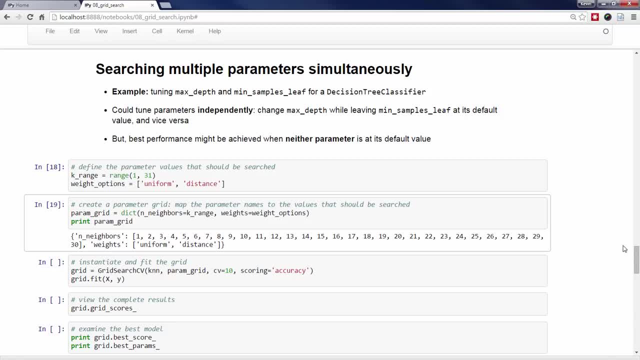 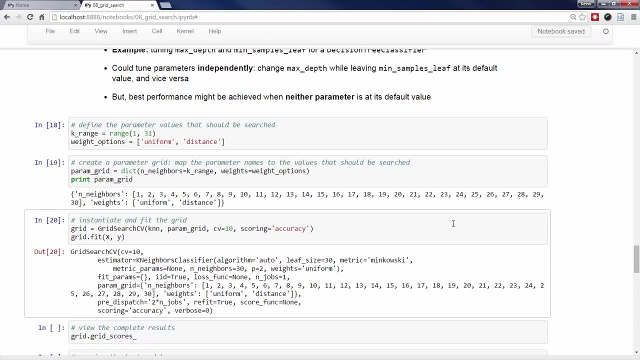 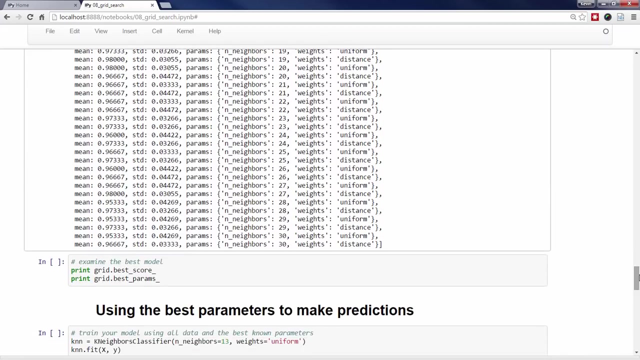 is being performed 60 times. Let's take a quick look at the results. You can see that there is a tuple for every possible combination of n, neighbors and weights. Once again, we'll examine the best score and the best parameters. Okay. 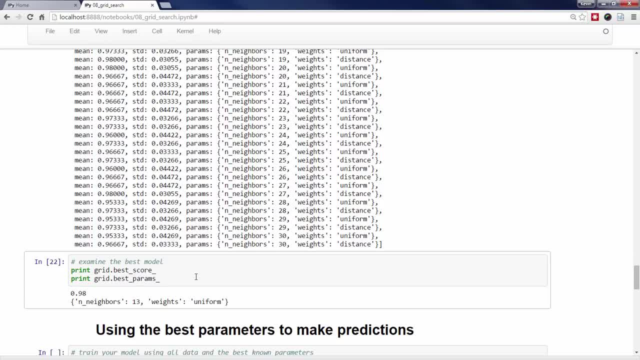 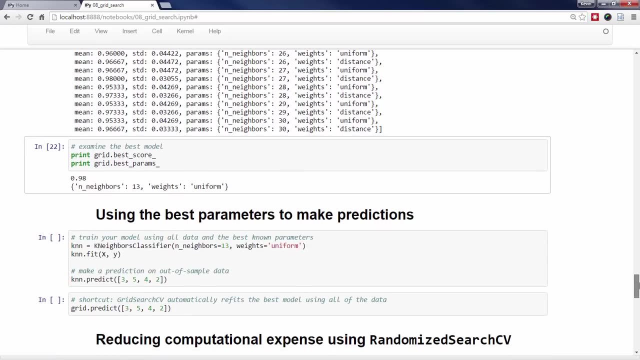 It turns out that the best score did not improve and thus, using n neighbors equals 13, with the default value for weights, is still the best set of parameters for this model. Next, I want to briefly remind you of what to do with these optimal tuning parameters. 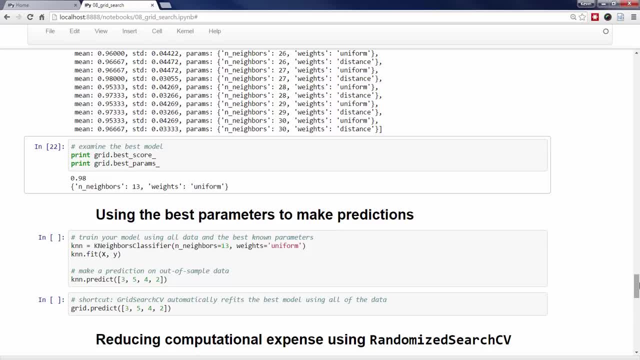 once you've found them Before you make predictions. Once you've taken the model out of sample data, it is critical that you train the model with the best known parameters, using all of your data. As you can see, I instantiate k-neighbors classifier with the best parameters I found. 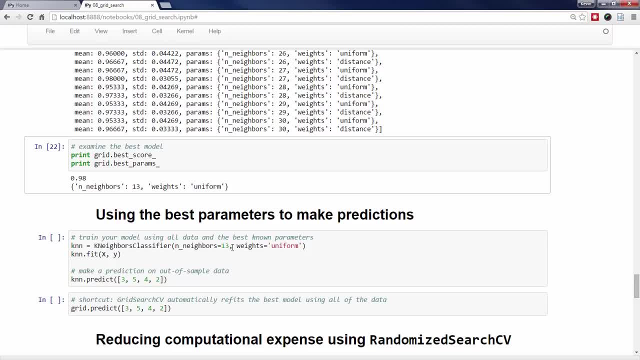 above and then fit it with x and y, not x train and y train. In other words, even if you used train-test-split earlier in the model building process, you'd still have to use the best known parameters for your model. You should train your model on X and Y before making predictions on new data. 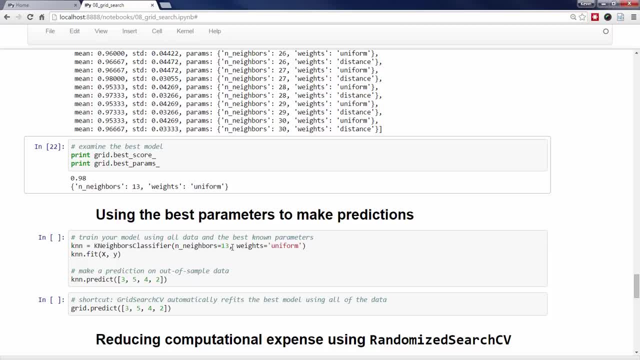 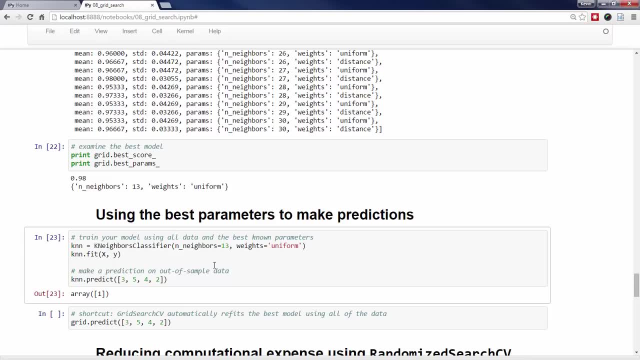 Otherwise, you will be throwing away potentially valuable data that your model can learn from. Here I've just made an example prediction on a made-up data point. However, GridSearchCV gives you a shortcut to this process. By default, GridSearchCV will refit the model using the entire data set and the best parameters it found. 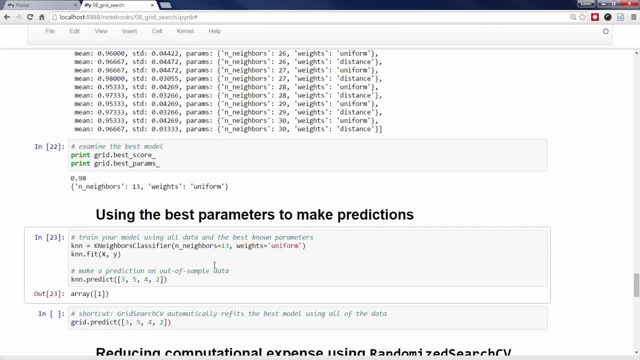 That fitted model is stored within the grid object and it exposes a predict method to allow you to make predictions using the fitted model. In other words, the code is stored within the grid object and the code in this cell accomplishes the same thing as the code in this cell. 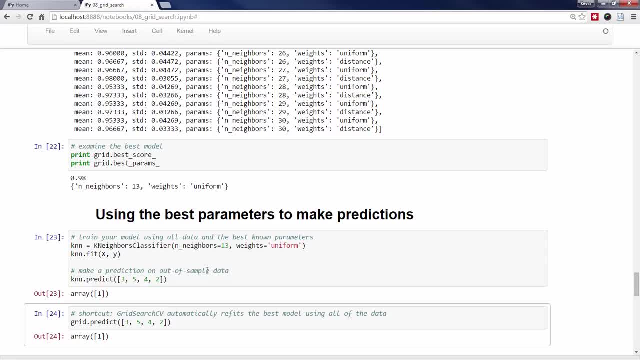 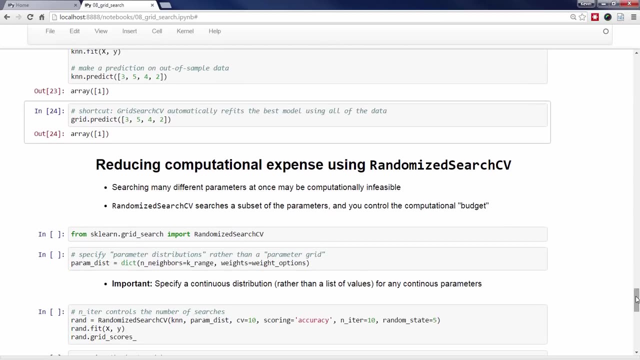 Obviously, this is only useful if you're running GridSearchCV right before making predictions, but it can be quite handy at times. Finally, let's take a look at randomized sort GridSearchCV, which is a close cousin of GridSearchCV. 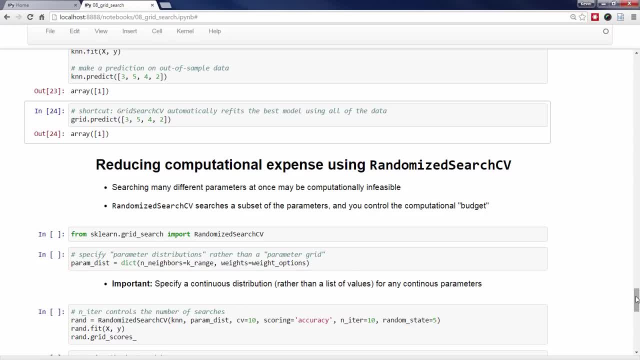 The problem that randomized search CV aims to solve is that when you're performing an exhaustive search of many different parameters at once, the search can quickly become computationally infeasible. For example, searching 10 different parameter values for each of four parameters will require 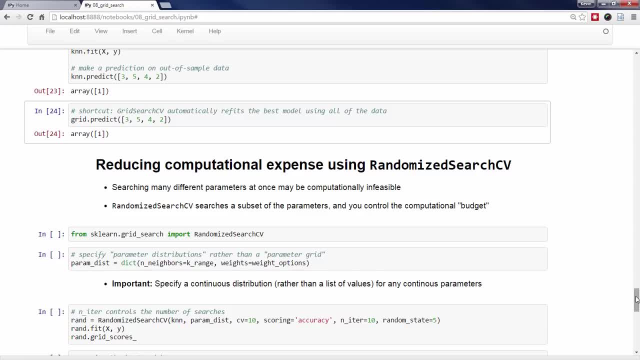 multiple trials of cross-validation, which would equate to 100,000 model fits and 100,000 sets of predictions if tenfold cross-validation is being used. Randomized search CV solves this problem by searching only a random subset of the provided parameters. 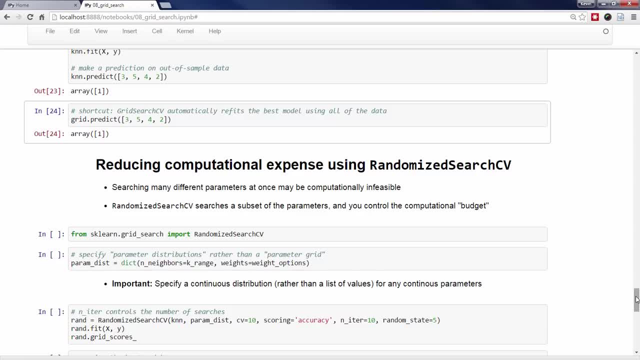 and allowing you to explicitly control the number of different parameter combinations that are attempted. As such, you can effectively decide how long you want it to run for, depending on the computational time you have available. As with GridSearchCV, we import the randomized search CV class from sklearngridsearch. 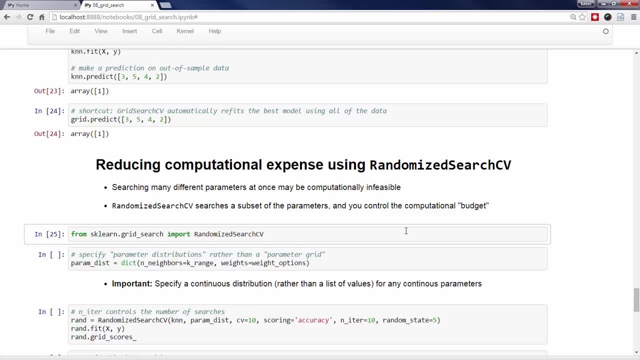 With randomized search CV, you specify parameter distributions rather than a parameter grid For discrete parameters, meaning parameters for which you provide a list of discrete values like integers or strings. this specification looks exactly the same as before. In this case, both of my parameters are discrete. 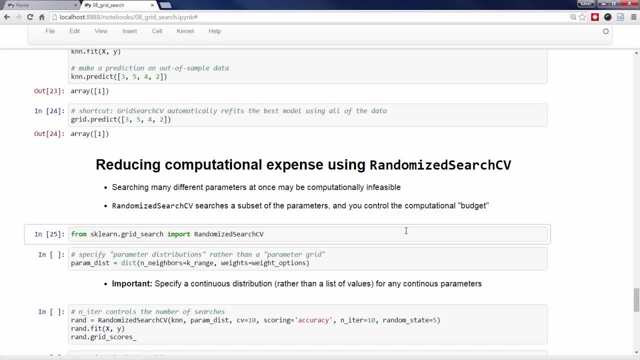 and so paramdist is no different from paramgrid. However, if one of your tuning parameters is continuous, such as a regularization parameter for a regression problem, it's important to specify a continuous distribution rather than a list of possible values, so that randomized search CV can perform a more fine-grained search. 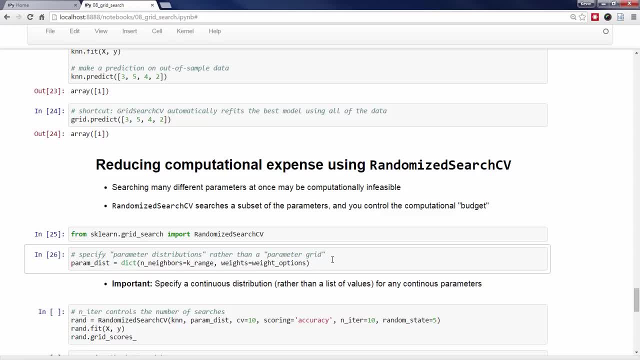 I don't have an example to show you here, but some of the resources I'll mention below include examples of this. Anyway, we can now instantiate the randomized search. fit it with data and take a look at the scores, You'll see that. paramdist. 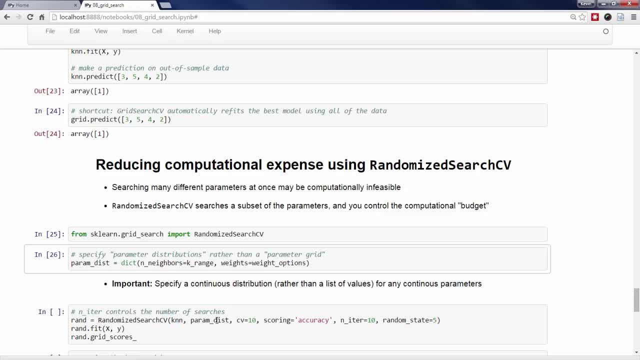 is used instead of paramgrid and there are two new parameters: niter, which controls the number of random combinations. it will try and randomState, which I've set for random, which I've set for the purpose of reproducibility. 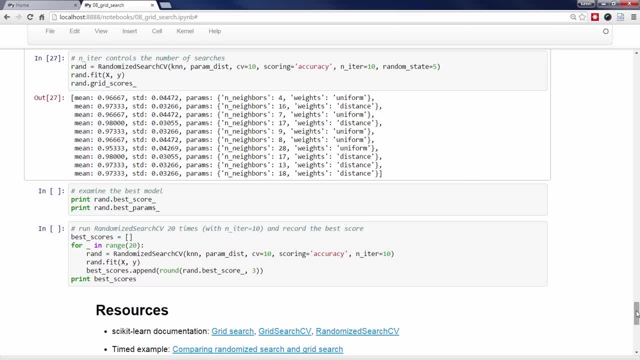 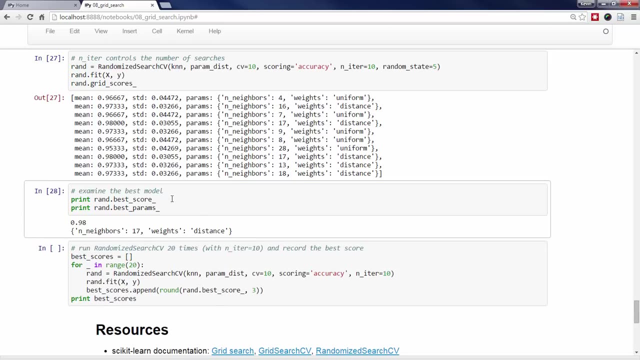 From the grid scores you can see that 10 random combinations of parameters were tried And once again we can look at the best score and the best parameters. We can see that, even though it only tried 10 combinations of n, neighbors and weights, 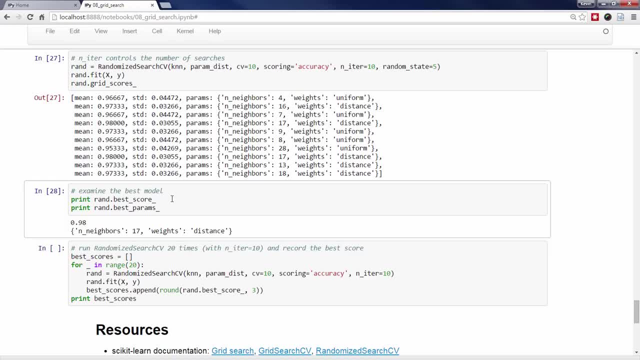 it still managed to find a combination that has just as high a score as the combination found by gridSearchCV. It's certainly possible that randomized search CV will not find as good a result as gridSearchCV, but you might be surprised how often it finds the best result. 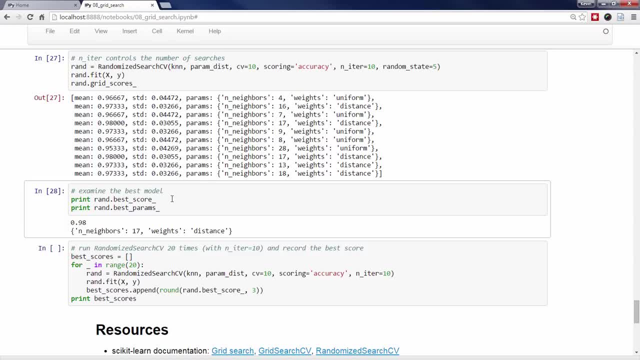 or something very close, in a fraction of the time that gridSearchCV would have taken. I've set up a quick experiment here in which I run randomizedSearchCV with niter equals 10, and I repeat this process 20 times. 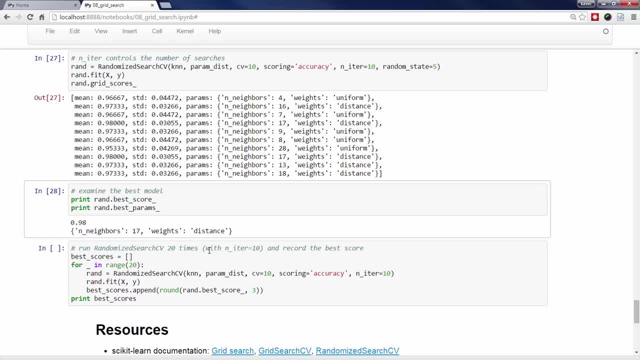 recording the best score each time. As you can see, most of the time it does result in a score of 0.98, and when it doesn't find that score, it's still close to 0.98.. In terms of practical recommendations,